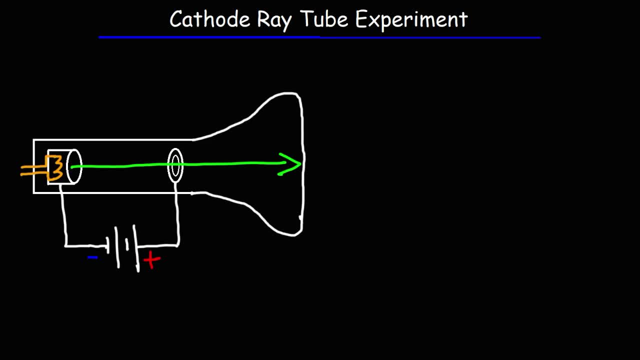 electron. So let's talk about the cathode ray tube experiment. So inside this device is an evacuated chamber. The pressure is very, very low. Most of the gas molecules have been removed such that the pressure is as low as 0.01 pascals At sea level. the pressure is one atm one. 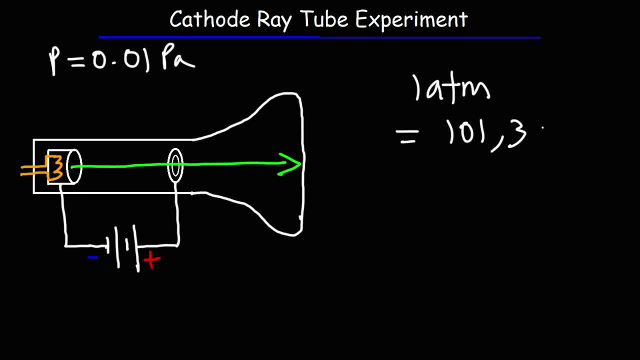 atmospheric pressure, which is equal to 101,325 pascals. So you can see the difference between the air pressure that we breathe and the very low air pressure inside of this evacuated chamber. If the pressure is too high, the electrons will collide with the gas particles and you won't get 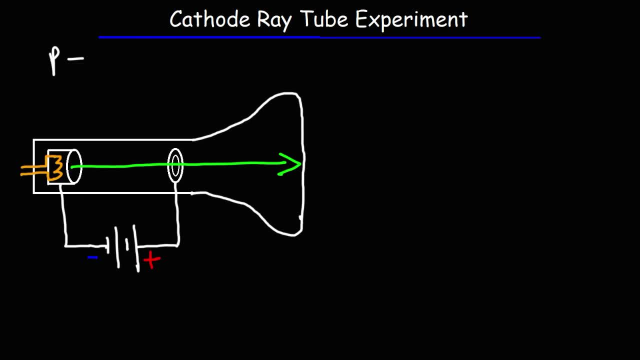 the same effect, It won't be visible. Now, inside the cathode ray tube we have something called a cathode and an anode. These are two different electrodes. The cathode is a negatively charged electrode and the anode is a positively charged electrode. 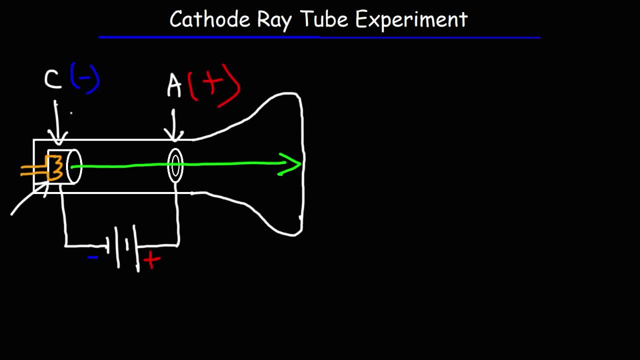 Now, when the cathode is heated by this heating element- nichrome wire is a good heating element. When it's heated and if there's a high voltage applied between the cathode and the anode, an electron beam is going to emanate from the cathode. 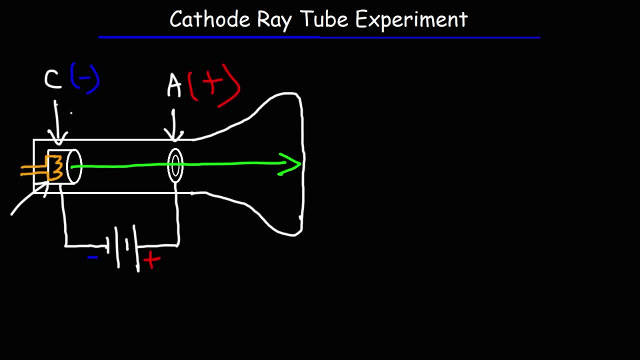 and it's going to accelerate towards the anode. Electrons are negatively charged, so they're attracted to a positively charged plate, So the anode accelerates this electron beam towards the right. So now the glass of this chamber is coated with a phosphorescent material known as zinc sulfide. 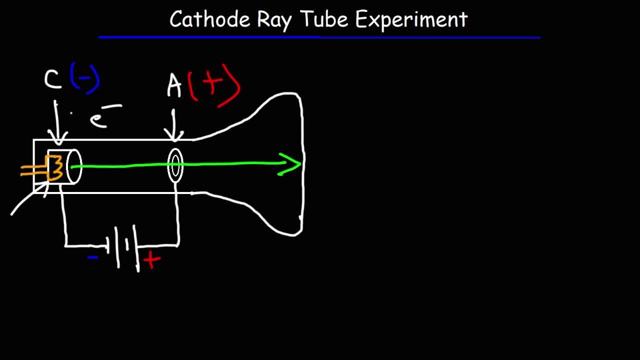 and so when the electrons strike the glass, they create this characteristic green glow, These cathode ray tubes, also known as CRTs. they were very useful in making TVs in the old days, Those big, large TVs. they contained the cathode ray tube device inside of it, And 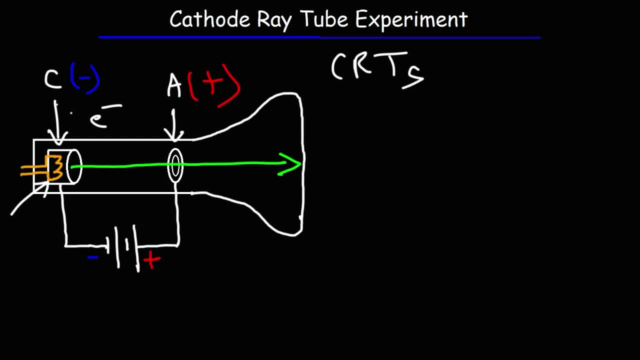 so when the electron beam strikes the screen, it will produce a characteristic image based on the on the voltage variant signal that is applied to it. Now here is a question for you. Why was this experiment called the cathode ray tube experiment and not the anode ray tube experiment? What would 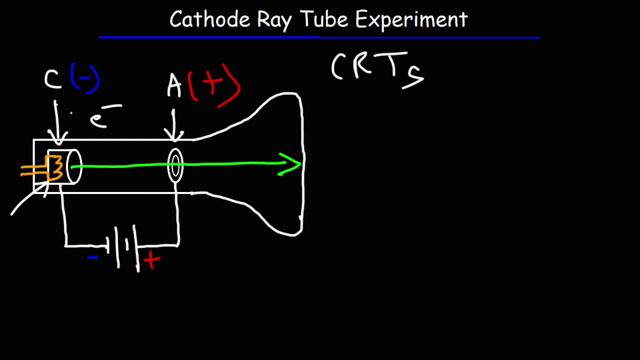 you say The reason for this is because the electron beam appears to emanate from the cathode and not the anode, and so it's called the cathode ray. Now here is another question to think about. What about this experiment helped JJ Thompson to conclude that all atoms contain electrons? 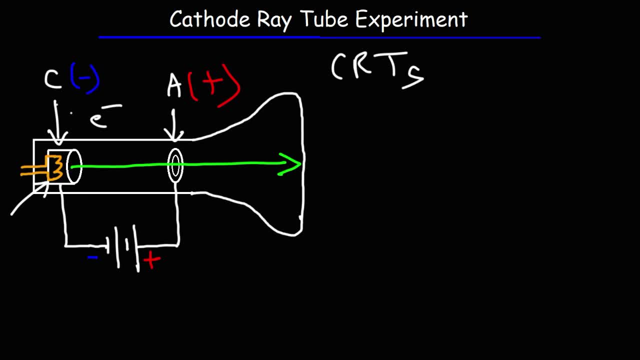 negatively charged particles. How did he determine that this beam consists of negatively charged particles? Well, the first thing is that this beam consists of charged particles because if you were to put a magnet next to it, the beam would deflect. A magnet will only deflect moving charges. It won't deflect stationary charges. so any object that is charged. 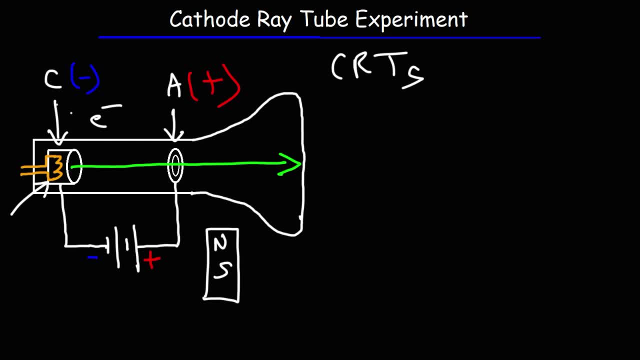 and is moving can be deflected by a magnet. The second thing is: if you apply- let me put a positively charged plate here and a negatively charged plate here- the beam will also be deflected, Would you say. it will deflect in the upward direction or in the downward. 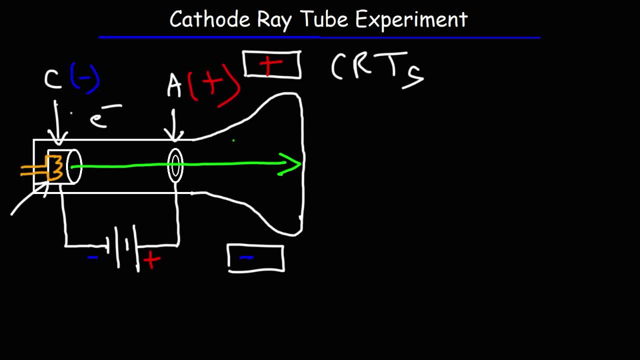 direction. What would you say? In this experiment the electron ray was deflected towards the positively charged plate. so therefore we know that opposites attract. That means that the beam must consist of the negatively charged particles. So that's how JJ Thompson came to the conclusion. 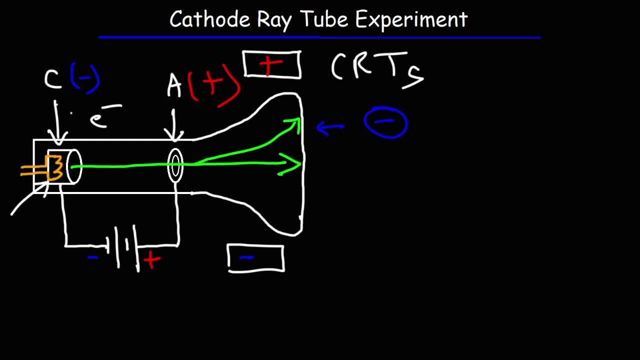 that this beam of particles consists of negative particles. So that is how JJ Thompson came to the conclusion that this beam of particles must be negatively charged. It's due to the fact that it was deflected towards the positively charged plate. Electrons are attracted to positive charges. 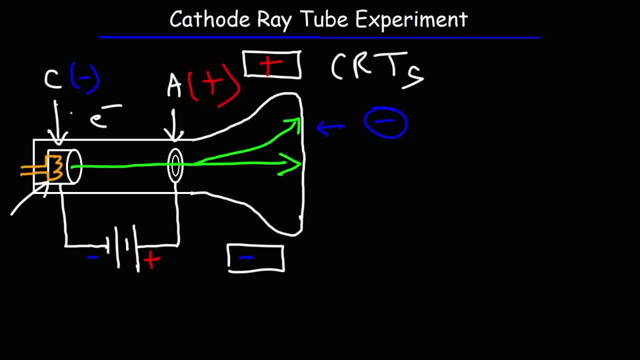 Opposite charges attract, as was mentioned before. Now, another thing that he experimented was with the use of different anode and cathode materials. It doesn't matter what metal the anode and the cathode were made of If we use zinc. 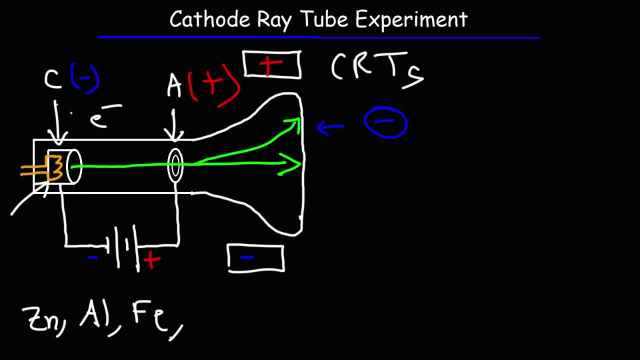 if we use aluminum, iron metal, copper, silver, all of these metals can emit a cathode ray. So the fact that these different metals can emit a cathode ray helped them to conclude that all atoms, not just certain types of atoms, but all. 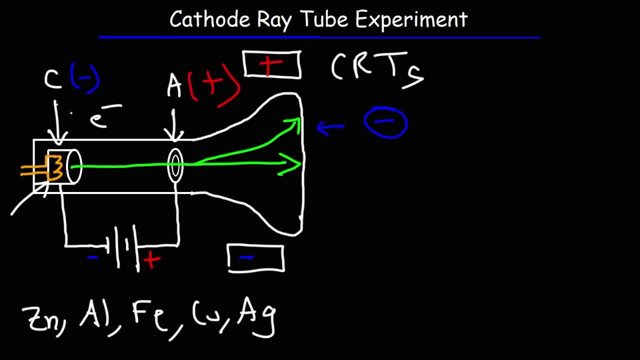 materials. all atoms contain negatively charged particles, which we now know as electrons. So now we understand how JJ Thompson was able to use the cathode ray tube experiment to determine the fact that atoms contain negatively charged particles known as electrons. But now what about calculating the charge to 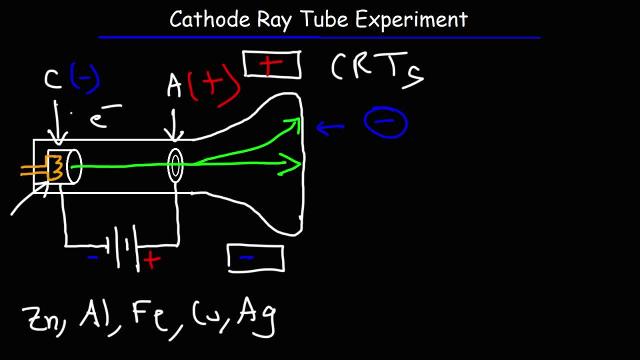 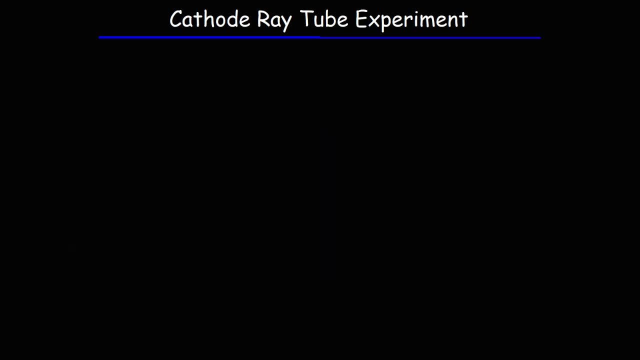 mass ratio of an electron. How did he use this experiment to get that number? Well, now we need to jump into the realm of physics. So let's talk about an electron. If we have a positively charged plate and a negatively charged plate, the electron will feel a force that will attract it or accelerate it towards a 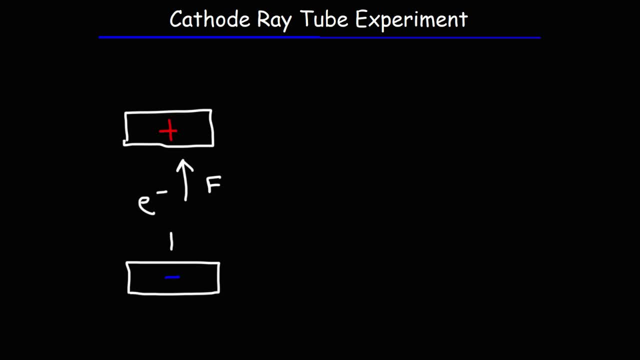 positively charged plate, It will also feel another force that will repel it from the negatively charged plate. So electrons can be accelerated by electric fields. They can also be accelerated by magnetic fields as well. A magnetic field can cause an electron to change direction. 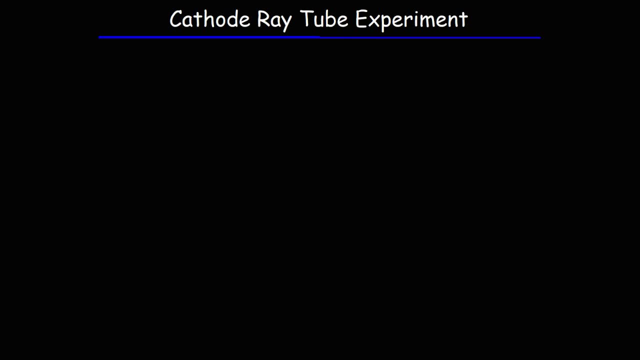 Not necessarily speed up, but it can accelerate it in a way that it can cause it to change direction. It could deflect it And we're going to talk about that. So let's say we have an electron that is moving towards the right. 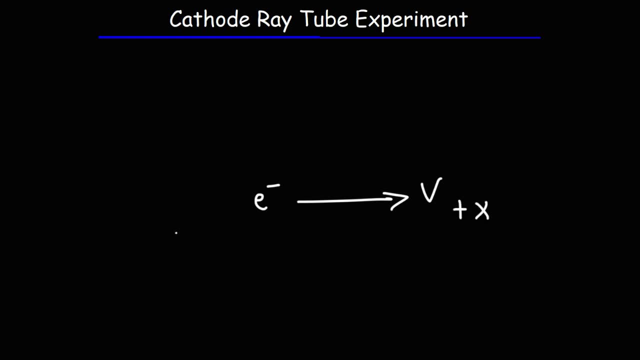 That is in a positive x direction And we have a magnetic field that is coming out of the page, The electron will feel a force that will accelerate it in the north direction, Or you could say in a positive y direction if you view it from a two-dimensional perspective. 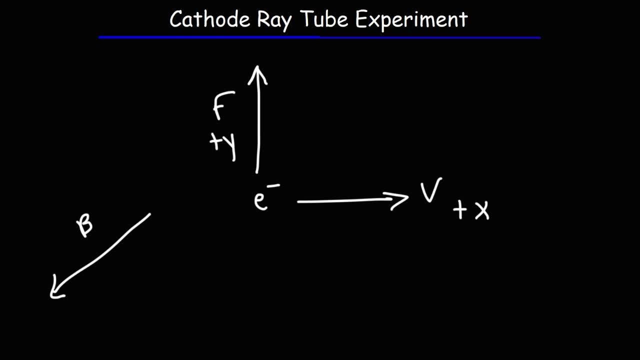 In a three-dimensional perspective, that would be the z direction. Now the electron is moving towards the right, But it feels a force that is accelerating it in that direction. Where will it go? In this case, it's going to turn. 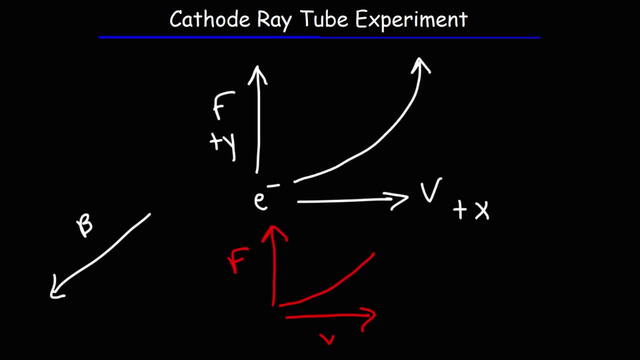 It's going to deflect in this direction And notice that you could extend this to make a circle. So by calculating the radius of curvature and knowing the strength of the magnetic field and the strength of the electric field, you can actually calculate the charge to mass ratio. 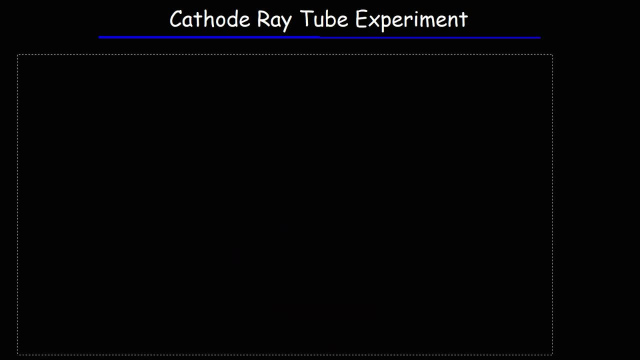 So let me make a new drawing with this. So let's say this point represents the electron, It's moving towards the right, So it has a velocity component in the positive x direction. The magnetic field is going to be. The magnetic field is represented by the symbol B. 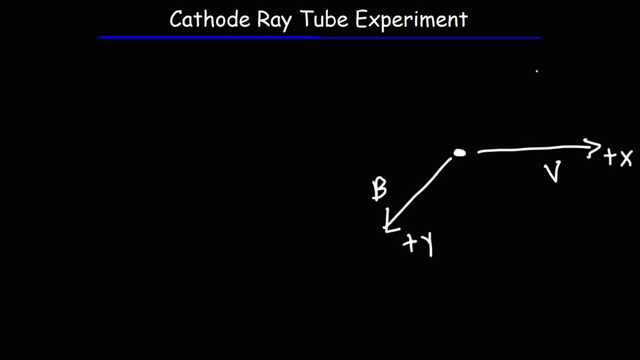 And it's going to be in a positive y direction from a 3D perspective. And the force, the magnetic force acting on the electron- Let's put F sub B to indicate magnetic force That is in the positive z direction, And so the electron is going to travel. 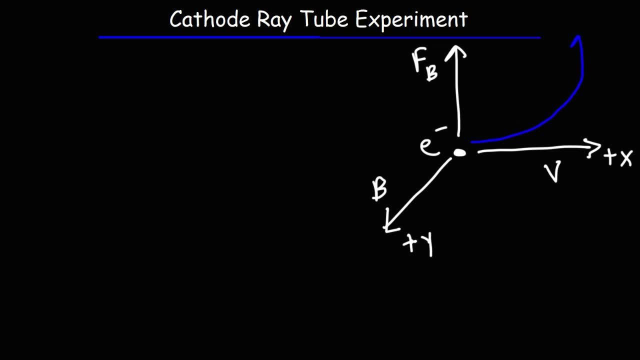 It's going to turn in the direction of the force, And then we can calculate the radius of curvature. So now let's go over some physics equations. The magnetic force, F sub B, that acts on a moving charge, not a stationary charge, but a moving charge. 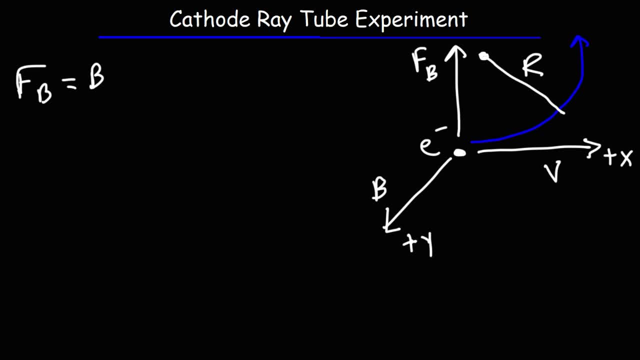 is equal to the strength of the magnetic field B, which is measured in units of Tesla, times, the charge of the electron, times the velocity of the electron. So if it's not moving, the velocity will be zero, The magnetic force will be zero. 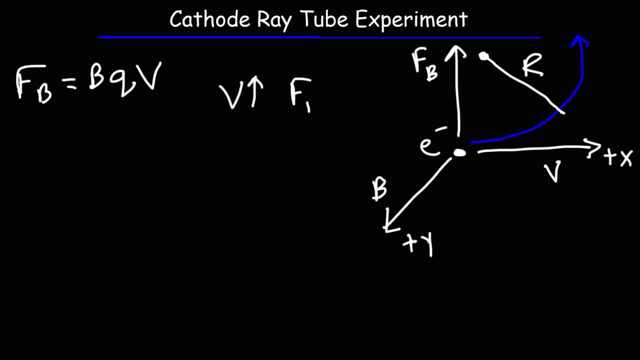 But as the speed of the electron increases, the magnetic force will be increased as well, proportionally, So you can increase the magnetic force. You can increase the magnetic force acting on an electron by increasing the electron speed or by increasing the strength of the magnetic field. 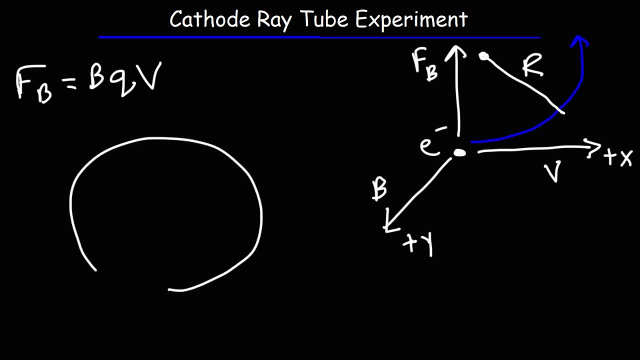 Now there's another type of force that occurs when an object moves in a circle, And this is known as a centripetal force. The centripetal force is not a force in itself. It is caused by another force that causes the object to turn in a circle. 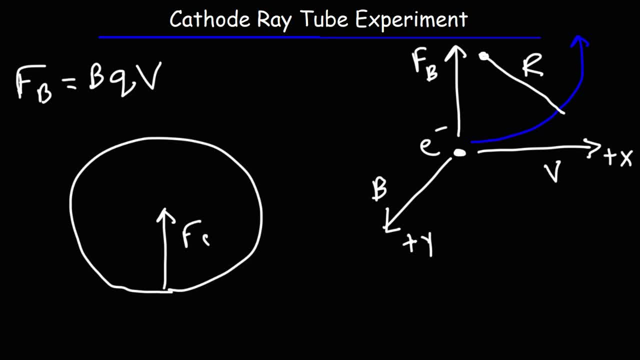 So if you think of how the moon orbits the Earth, it provides a centripetal force. in that case, In the case of the electron turning, the magnetic force provides the centripetal force. So any force that causes an object to move in a circle. 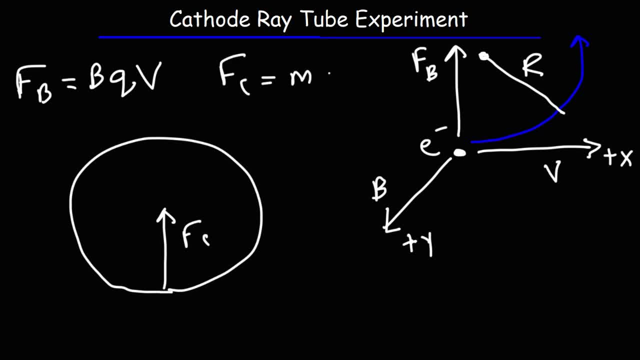 is a centripetal force And it's equal to mv squared over r. So because the magnetic force provides the centripetal force in this example, we can set these two forces equal to each other. So we could say that bqv is equal. 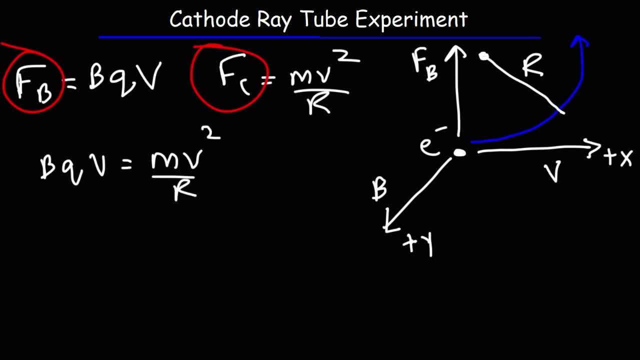 to mv squared over r. If we divide both sides by v, we're going to get: bq is equal to mv over r, where m is the mass of the electron, v is the speed or the velocity of the electron and r is the radius of curvature. 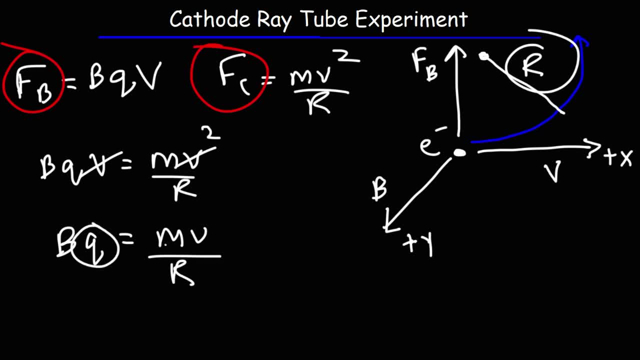 So to get the charge-to-mass ratio we need to get q over m. So I'm going to multiply both sides by 1 over b and also by 1 over m. So on the left, b is going to cancel, On the right, m is going to cancel. 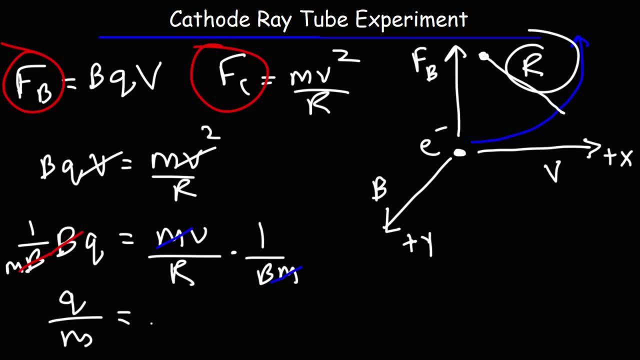 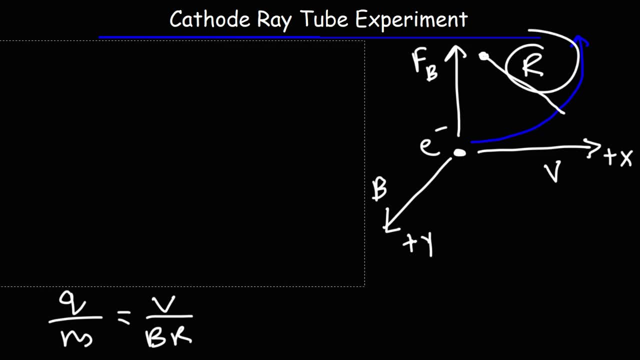 So q over m is equal to v over b times r. q is the charge of the electron, m is the mass of the electron, v is the speed, b is the strength of the magnetic field and r is the radius. Now we can easily determine. 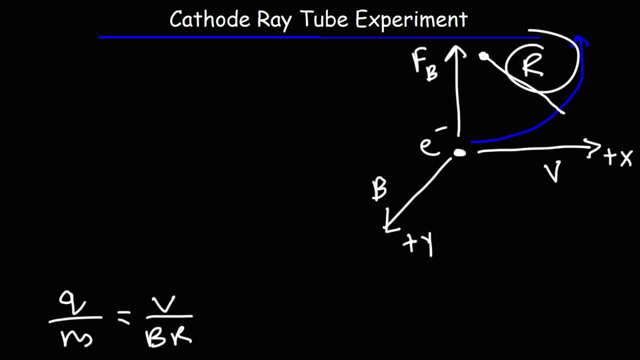 the strength of the magnetic field, because we can control the amount that we apply in the experiment And we can measure the radius of curvature. But measuring the speed of an electron is not going to be easy to do, And so we need to remove it from the equation. 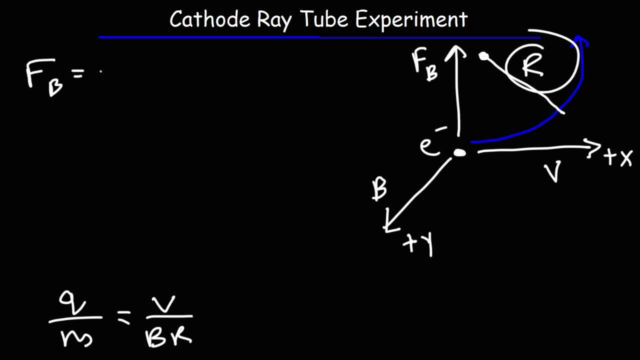 The magnetic force acting on a moving charged particle, as we said before, is equal to bqv. The electric field, or rather the electric force acting on any charged particle, regardless if it's moving or if it's stationary, is equal to the charge of that particle. 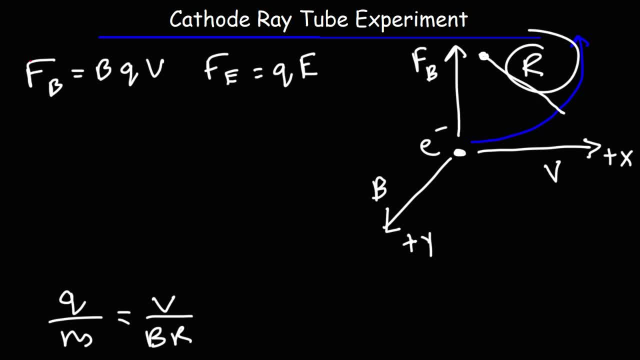 times the electric field. Now what we need to do is we need to set this experiment in such a way that these two forces are equal and that they cancel out. If we can do that, then we can set bqv equal to q times z. 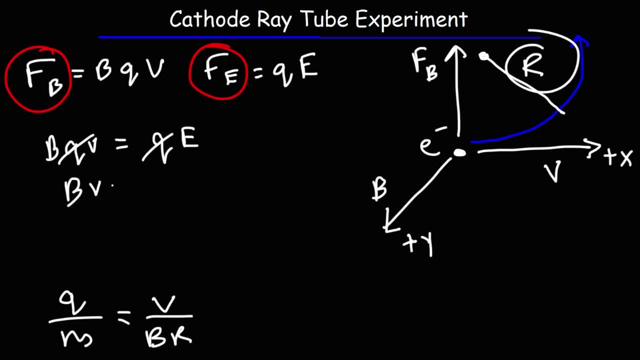 Dividing both sides by q, we get b times v is equal to e, and dividing both sides by b, we get that the speed of the electron is equal to the electric field divided by the magnetic field. If we design the experiment in such a way, 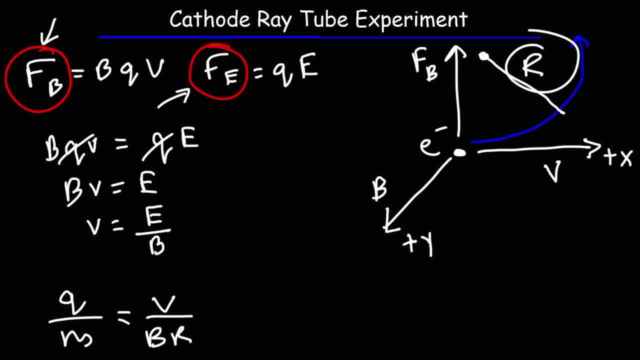 that these two forces are equal. So we can replace v with e over b. So we have: q over m is equal to 1 over b, times r and then times v, which is e over b. So the charge divided by the mass. 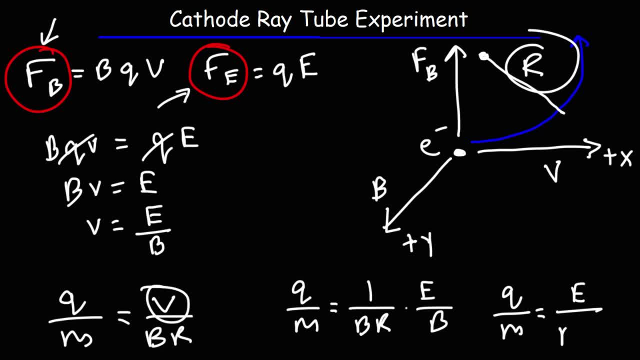 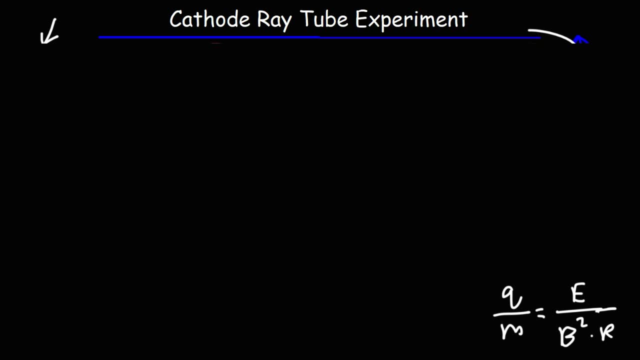 is equal to the electric field divided by the square of the magnetic field times the radius of curvature. So let me show you how we can set this experiment up such that the magnetic force cancels the electric force. So let's say we have two plates. 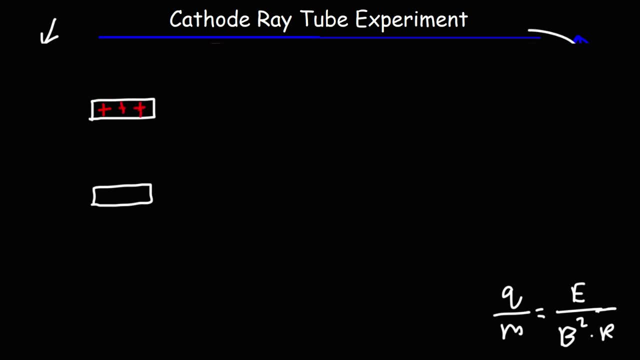 One is positively charged and the other is negatively charged, And let's say we have an electron beam that is traveling in this direction. There's going to be an electric field that emanates from the positively charged plate and flows towards the negatively charged plate. 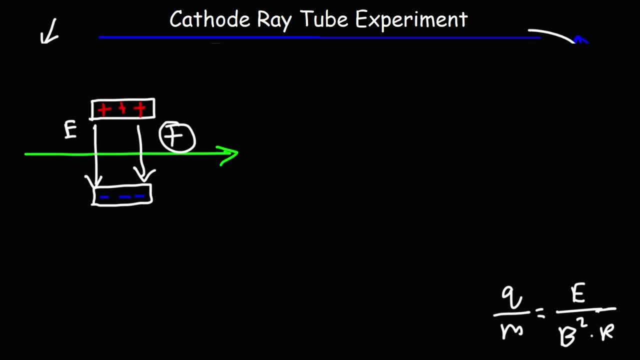 Now a positively charged particle, like a proton, will feel a force, an electric force that will accelerate it in the direction of the electric field. In this case, it will accelerate towards the negatively charged plate. A negatively charged particle, like an electron, will feel an electric force. 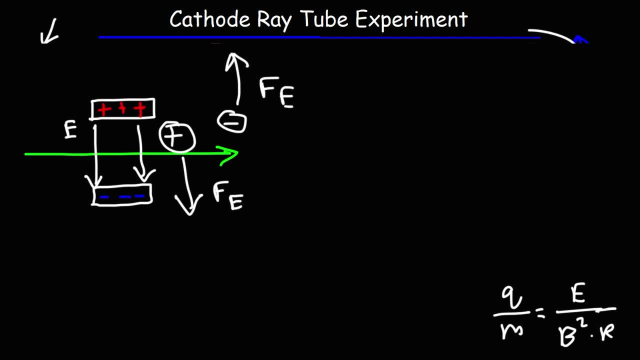 that will accelerate it in the other direction, that is opposite to the direction of the electric field, and so it's going to be accelerated towards the positively charged plate. So the electrons in this electron beam, they will want to deviate towards the positively charged plate. 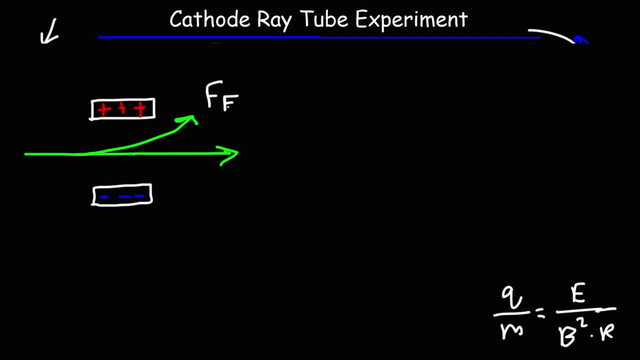 And this is due to the electric force acting on them. Now, if we have a magnetic force that is directed into the page, using the right-hand rule you could determine the direction of the magnetic force on the electron. So let me see if I still have my 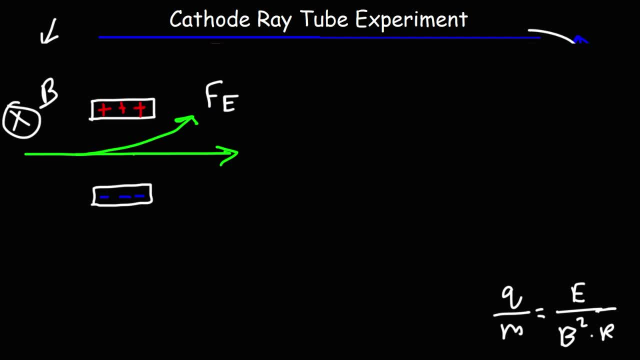 drawing skills. So what you want to do is using your right hand. you want to place your four fingers into the page and your thumb you want it directed in the direction of the electrons, So you want your thumb pointing towards the right. 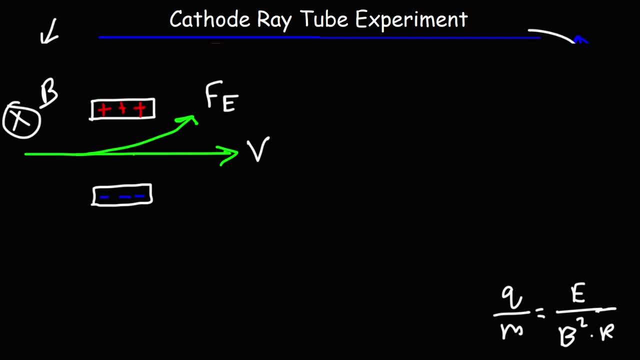 your four fingers pointing into the page, Your right hand should be opening in the upward direction. The magnetic force will be in the upward direction for a positively charged particle, But for a negatively charged particle it's going to be in the opposite direction. 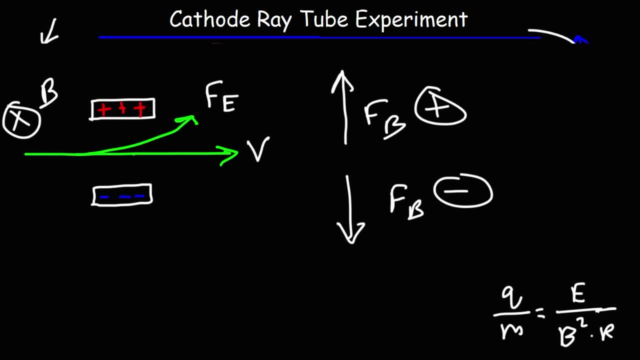 using the right-hand rule. Now, if you want to learn how to use it, there's a video that I created on YouTube. So if you go to right-hand rule- I mean, let me say that again- If you go to YouTube- 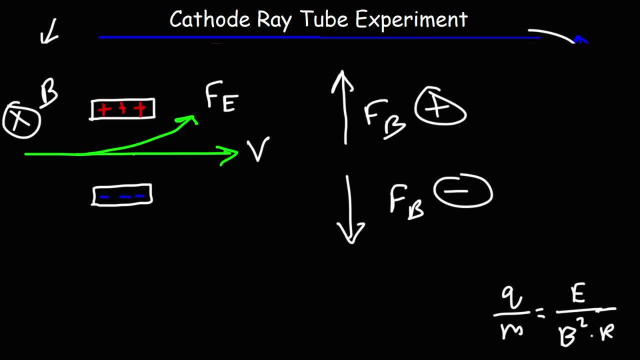 and type in the search bar right-hand rule: organic chemistry tutor. you'll find it And it could show you how to determine the direction of a magnetic force on a moving charged particle. But what you need to know is that when the magnetic field, 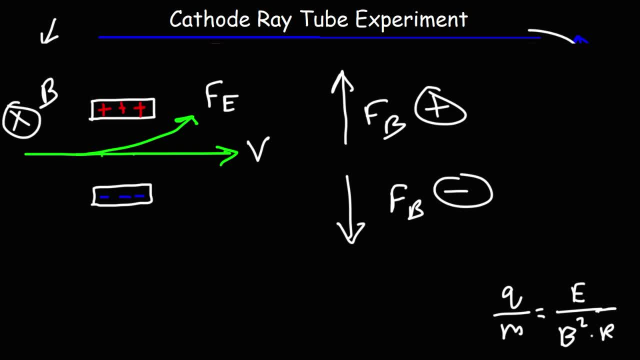 is directed into the page, the electrons will fill a force that will direct them this way, Due to the magnetic force. Now, if we can design the experiment in such a way that these two forces are equal, they will cancel out, And so the electrons will continue. 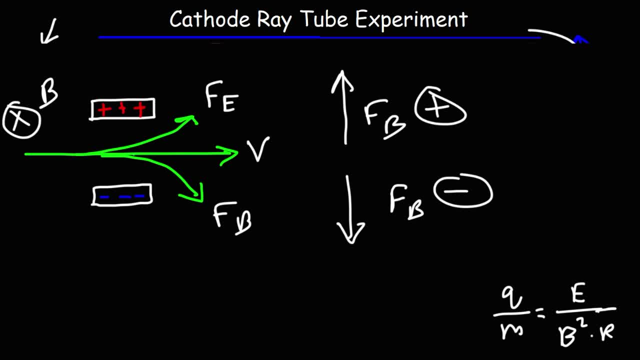 to move straight to the right, And so that's why we could set FB equal to FE to get this equation. It all depends on if we can balance those two forces. If we could, then we can calculate the charge to mass ratio using this formula. 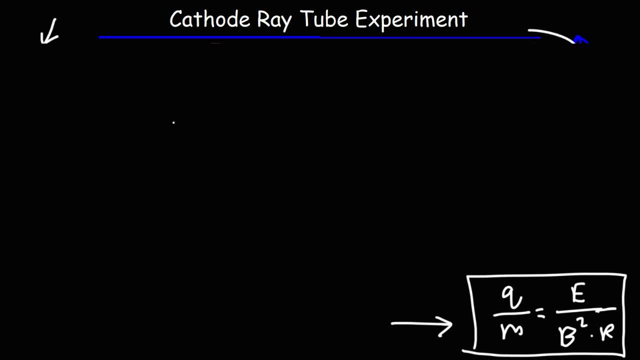 So now, once the beam of electrons passes through the electric field, what's going to happen is it's going to turn, Because the magnetic field is still active everywhere. Now let's say we have a material here. What's going to happen is: 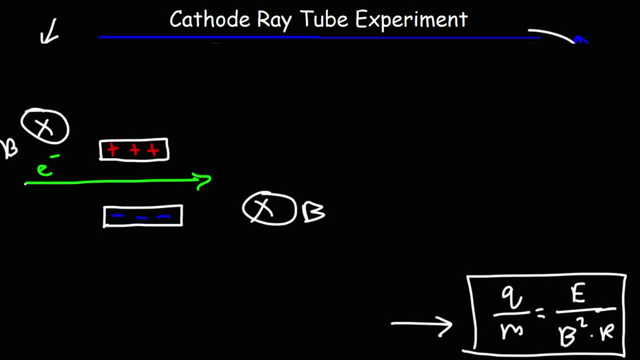 once it escapes from the electric field- and the magnetic field is the only force acting on it- it's going to turn And it's going to hit somewhere along this spot, And then we can calculate the radius of curvature. So now we know the strength. 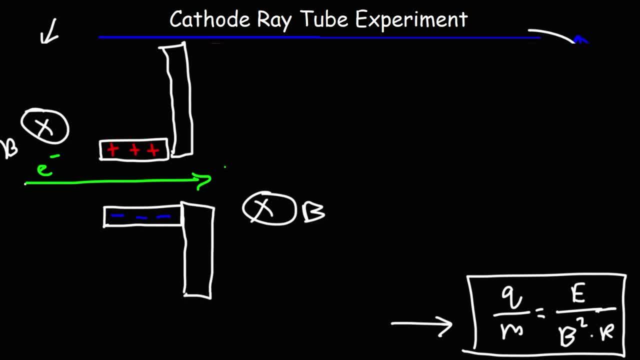 of the electric field that we're applying. The strength of the material that we're applying is going to be the force acting on it, So we can calculate the radius of curvature. So now we know the strength of the electric field that we're applying. 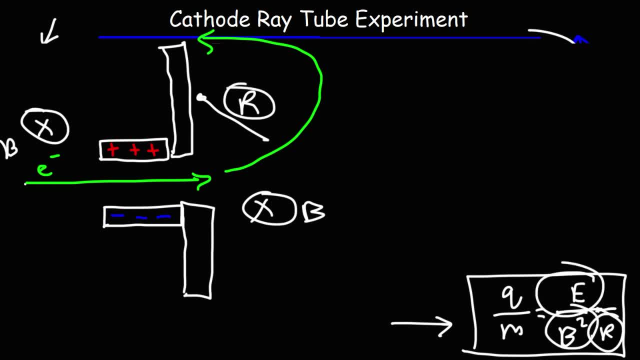 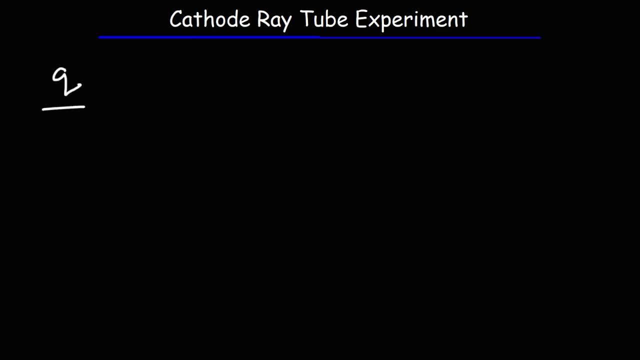 The strength of the magnetic field and the radius of curvature, We can now calculate the charge to mass ratio. So JJ Thompson discovered that the charge to mass ratio of an electron is negative: 1.76 times 10 to the 8.